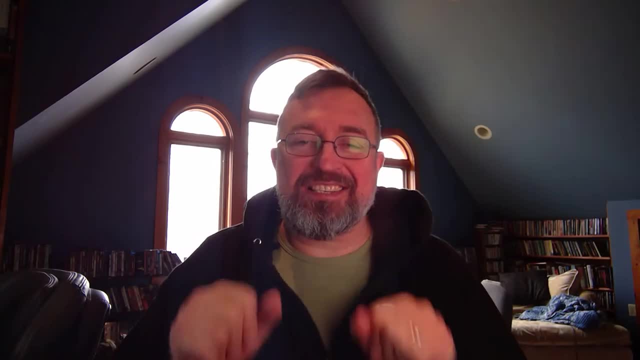 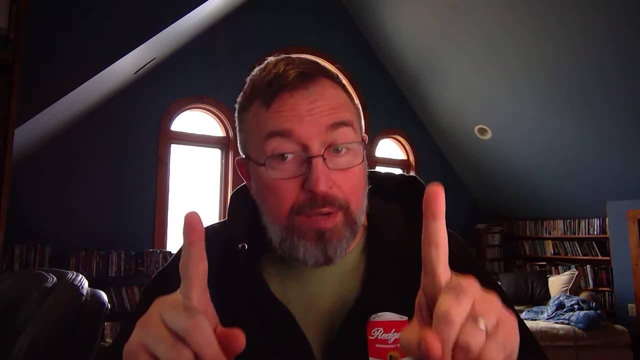 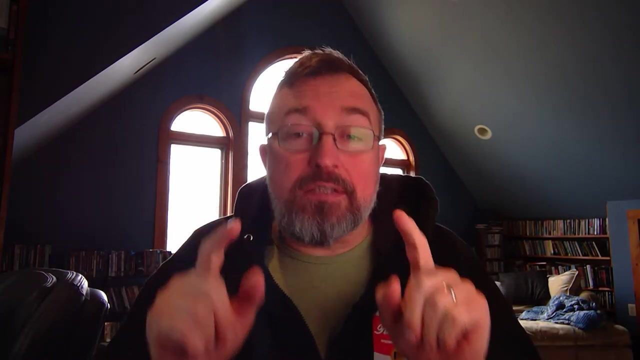 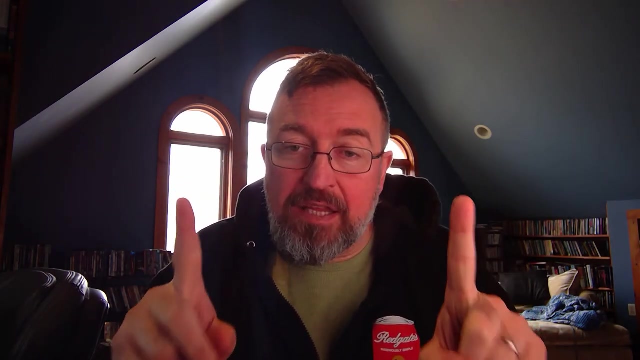 So let me tell you what the actual answer to this is. First, a block is when a resource is needed by two processes and one must wait on the other. That's a block Done. A deadlock is when we have two processes. Each is holding a process that the other needs. 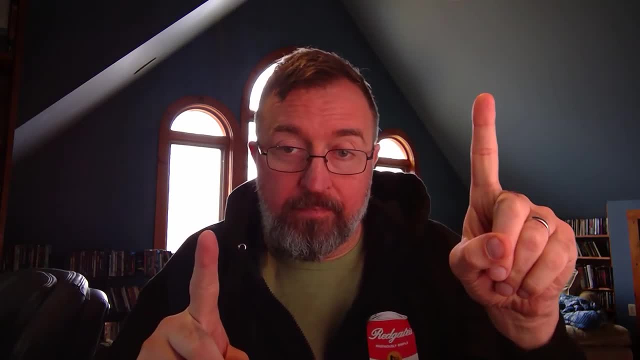 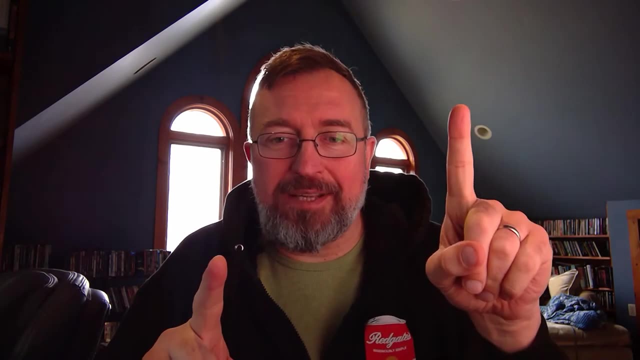 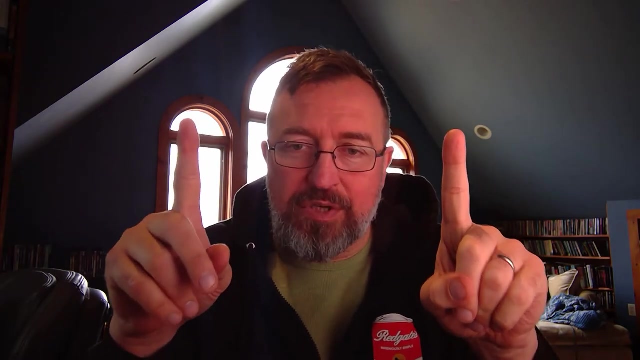 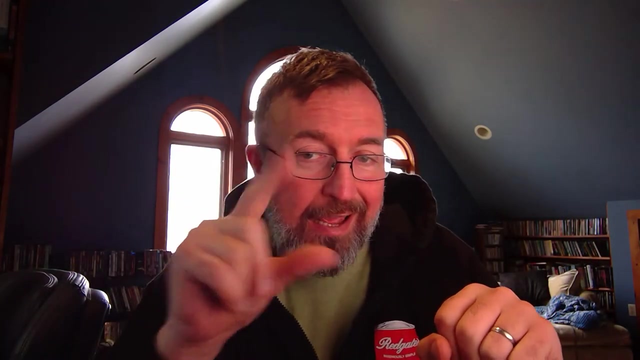 Process 1 has resource A and resource Z- I'm sorry- resource A and needs resource Z. Process 2 has resource Z and needs resource A. Okay, These two. I can't release Z until I get A. I can't release A until I get Z. 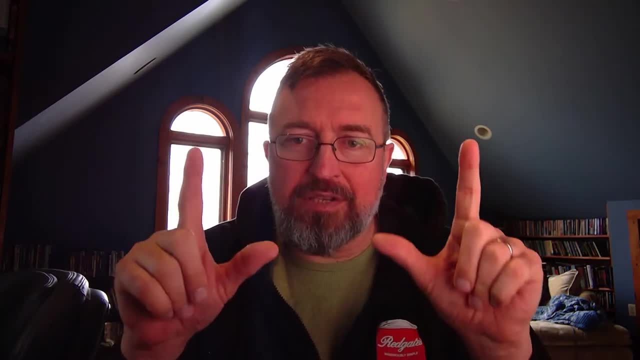 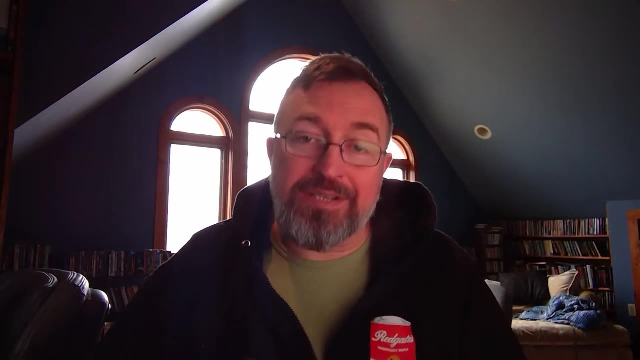 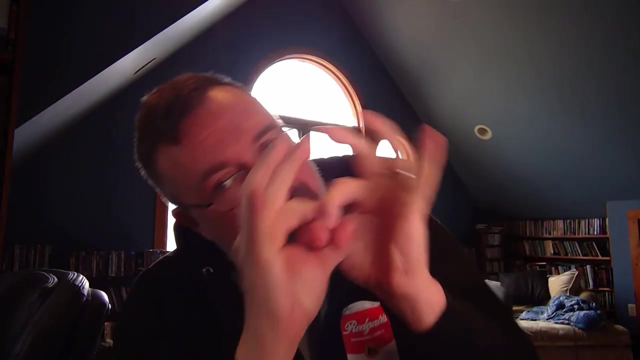 They are in a deadlock because of that deadly embrace, okay, That is a deadlock situation. There's a process inside of SQL Server that monitors for deadlocks and as soon as it sees that, hey, here are these two processes. they are intermingled in a way that they can never untangle right. 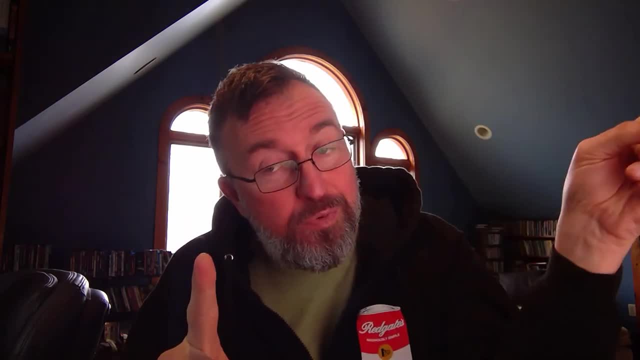 It's not like a block where it's like I'm waiting on this and as soon as it releases, I get to go. It doesn't matter how long that is, I can wait. right, It's all safely, I can wait. 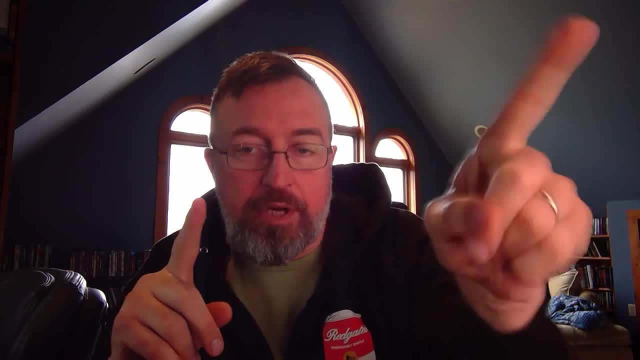 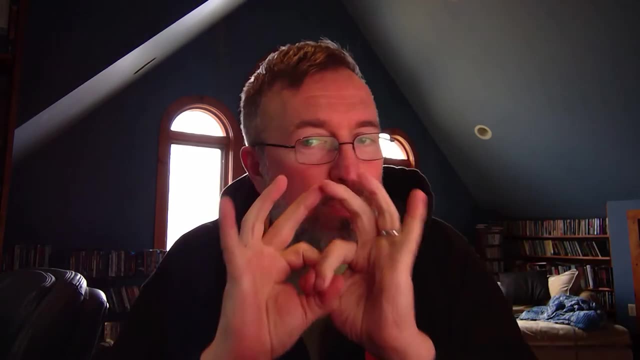 If that's four hours, four days, four weeks, four months or four years, I'll just wait until that releases and then I'll go. That's a block, The deadlock. they will never, ever, ever, ever release. 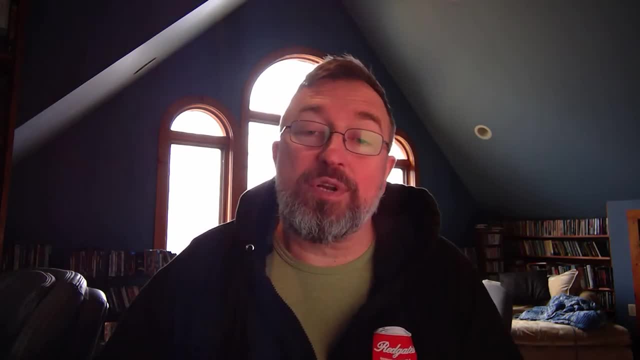 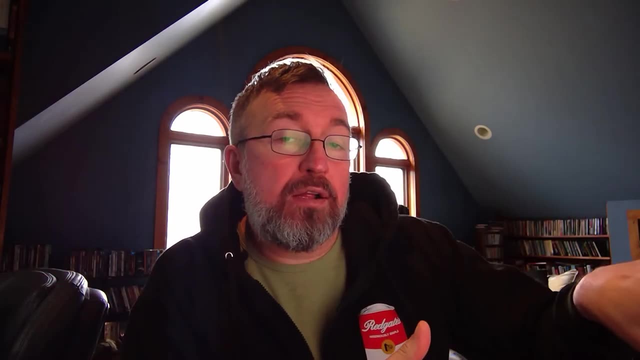 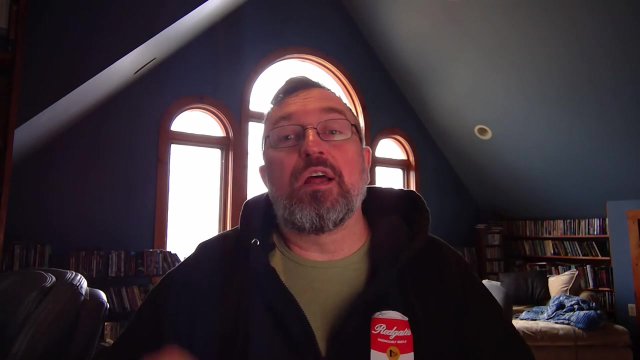 The process inside of SQL Server identifies which of these things is going to be the easiest to roll back, and then, da-da-da-da, It rolls back the easiest process because it has been chosen as a da-da-da-da. deadlock victim. okay, Now you know the answer to one of my favorite interview questions. 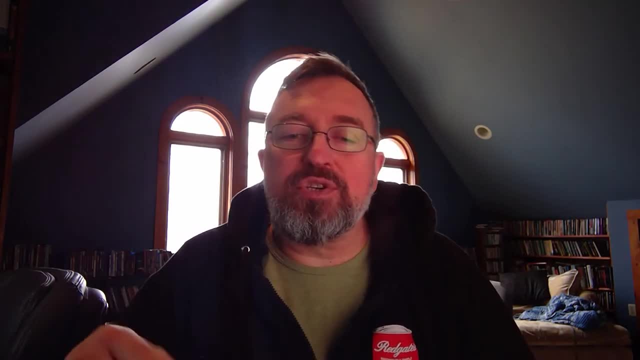 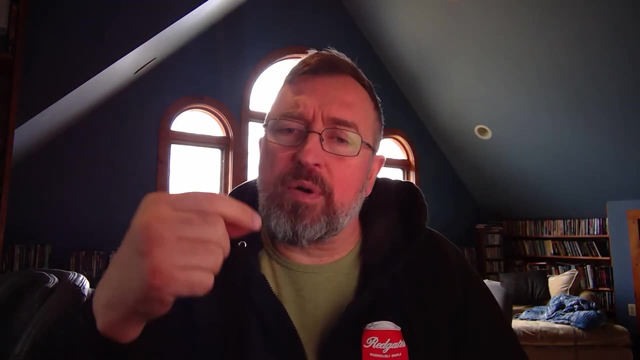 Cool. Now. deadlocks are a big issue. They're a major performance problem and we need to monitor for them and keep an eye on them and know how to observe what they are and figure out where the two resources are that are causing our deadlock. 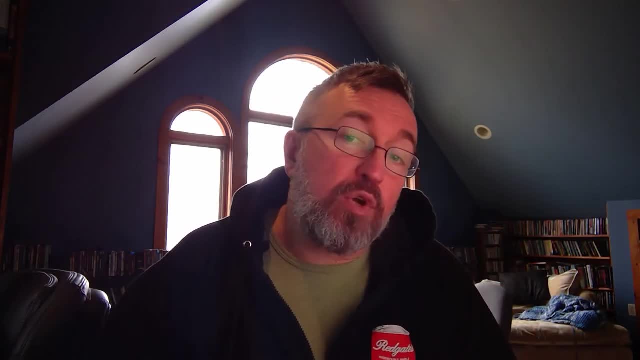 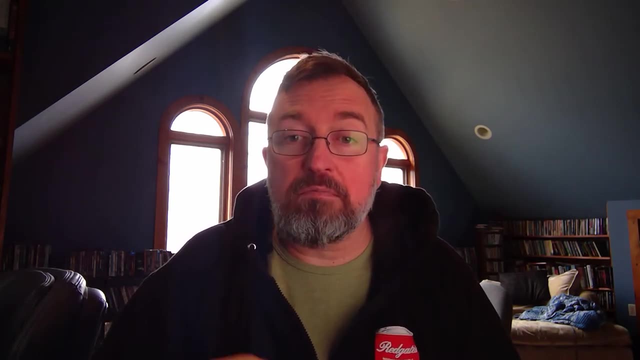 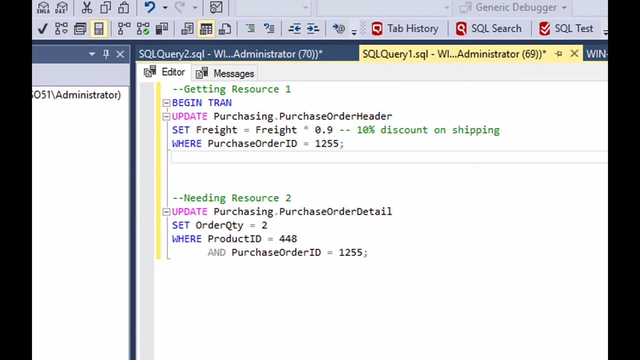 Why are we getting a deadlock? Let's go look at this example of using SQL Monitor from Reggeit Software to deal with deadlocks. So this is Management Studio, This is T-SQL, And I'm going to put together a deadlock for you guys right now. 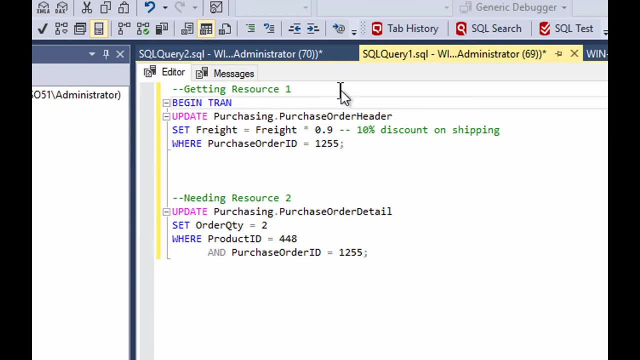 So what we're going to do is we're going to go over here to resource number one and we're going to run this query and this is going to take a lock-out. It's going to try to update some data, So it's going to take locks out. 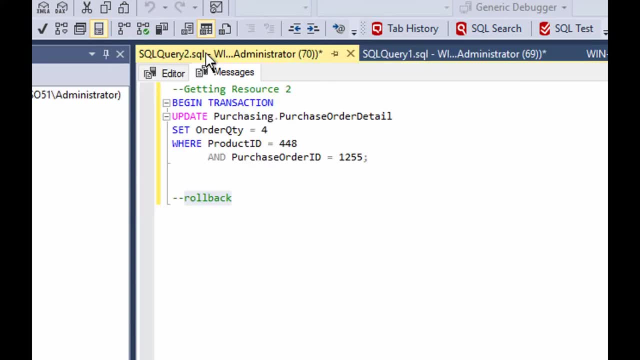 on a query and that's run successfully. it opened a transaction and got going. now we're gonna go over here to this other connection- a completely different connection, same database- and we're going to start another transaction of this transaction needs the resources of the transaction that we've already started. 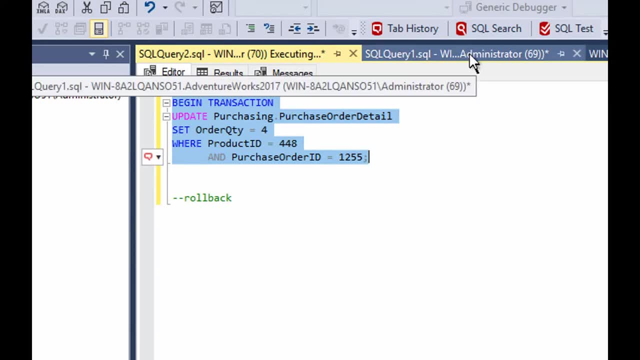 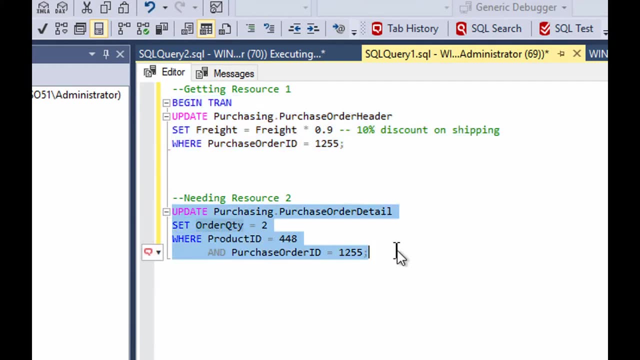 so you'll see it's executing and waiting. this is a block, right, this is being blocked. now let's change and run a second command over here, because we've still got an open transaction. right, we've got the begin Tran. we haven't committed a rollback, so this is still an open transaction. let's execute another. 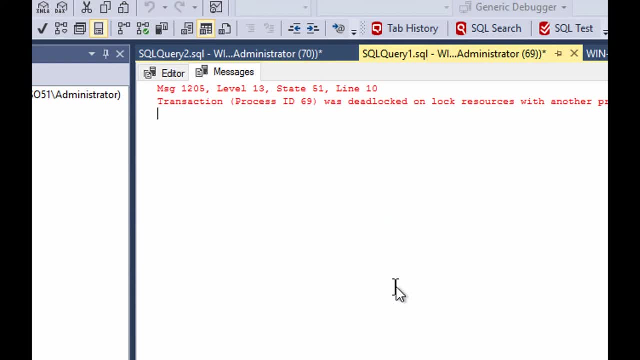 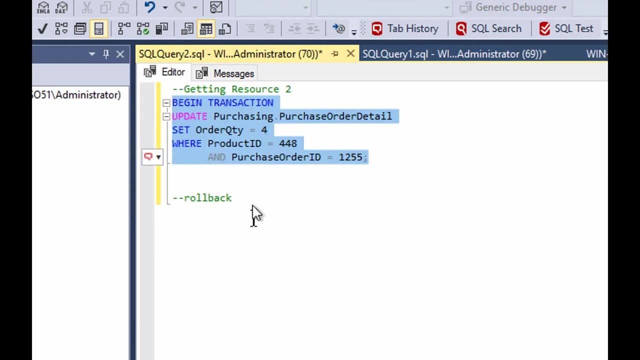 query. now this is going to update different data and tada, this query was chosen as a deadlock victim. rerun the transaction and you'll notice that this first query- I'm sorry, the second query over here- has now completed and it's good to go now, just in order to maintain my data sets and stuff. let's just roll. 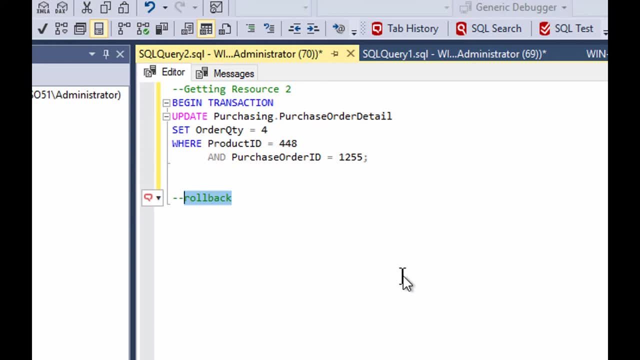 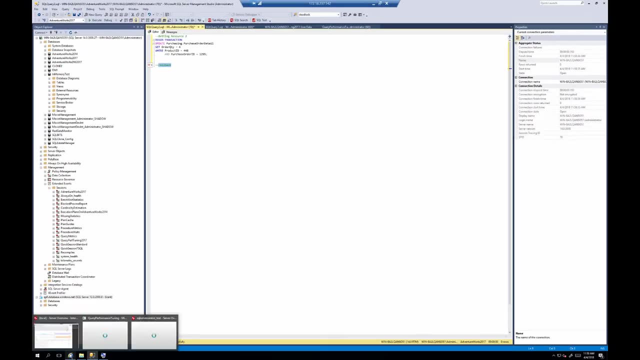 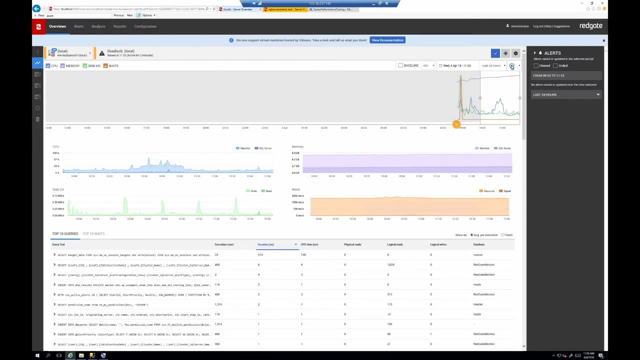 this up back. that's not something you need to worry about normally. normally that transaction completes and everything's happy. but I'm just doing that for for demo purposes. so now what's gone on is, if you take a look over here at SQL monitor and we refresh to show that we're on the latest time, we received a. 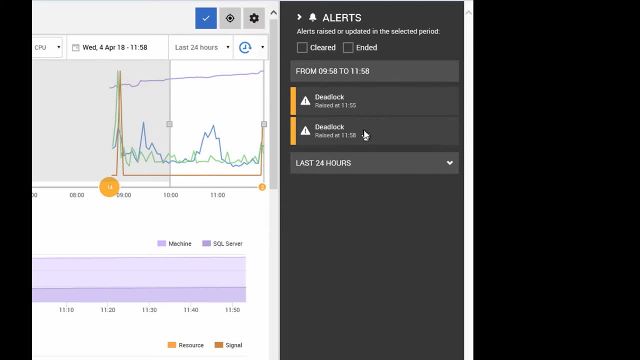 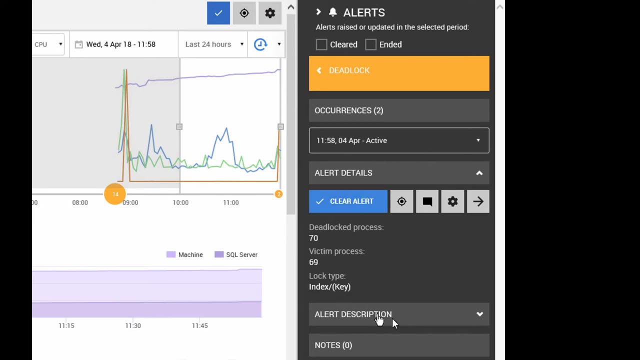 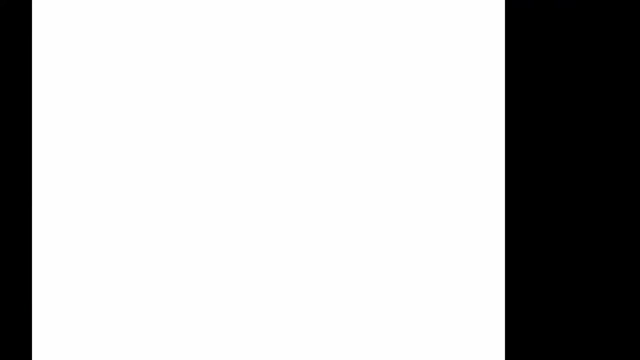 deadlock and so we can click on this and it will show us the alert and so we can see what's going on and it and it's done a deadlock, you know there's some. let's take a look at the description. there's a deadlock raised, you know. let's see more information and 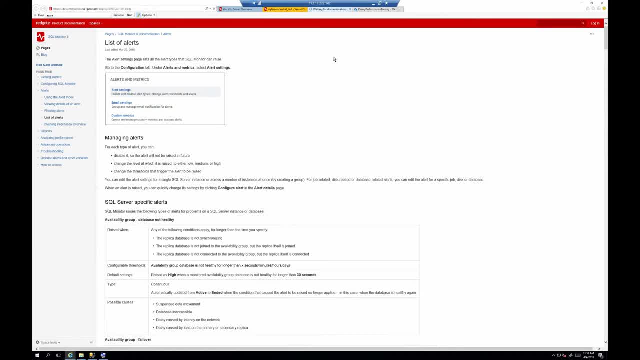 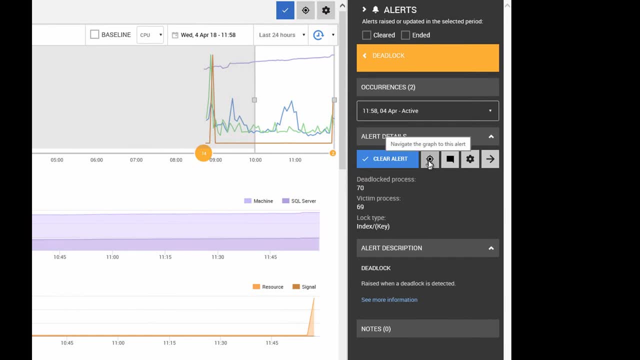 this tells us all about. you know what happens for specific alerts and and what they mean. great, but really what we need to do is drill down on this thing to understand what's going on so we can navigate the graph directly to win. the alert occurred and so it takes us to win. that moment in time occurred and we can see it here. 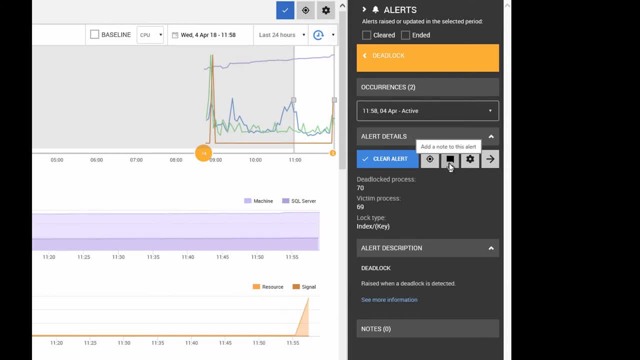 as well. we've got two alerts going on. we can add a note to the alert to mark off what this is, why it happened- all that kinds of fun stuff. we can go and configure the alert or, best of all, we can go to the full alert details. 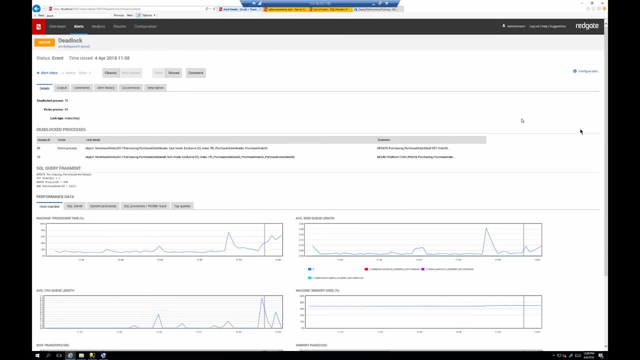 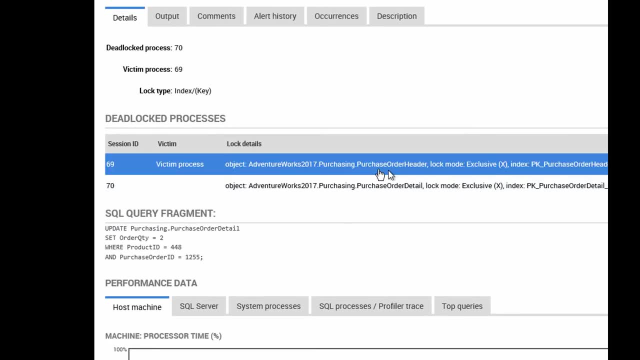 let's take a look at that. and so now what we get is we start to see information so we can see that there was the object that was taken exclusively lock on, and then the victim process what lock it was attempting to take a lock on, and you'll notice that you know, you can see which query was running and which. 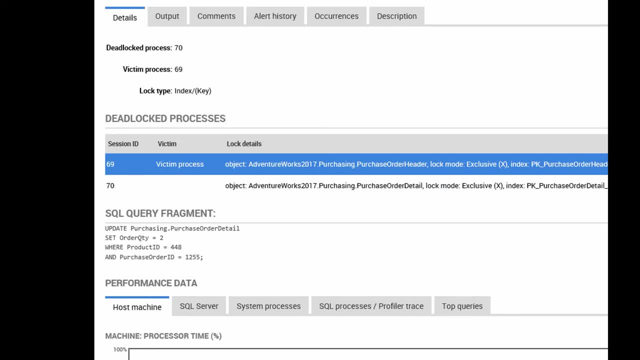 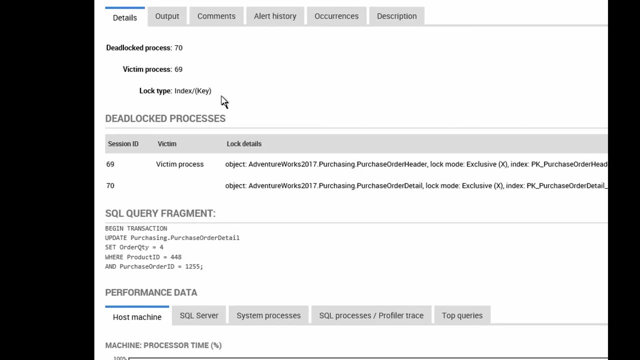 query was running here. each of these things can be drilled down on to get further information, and so we've got the information, the process that was done, the victim process, what types of locks, exactly which query fragments they were in, so you can track all of this down. you can go and look at some of the details. 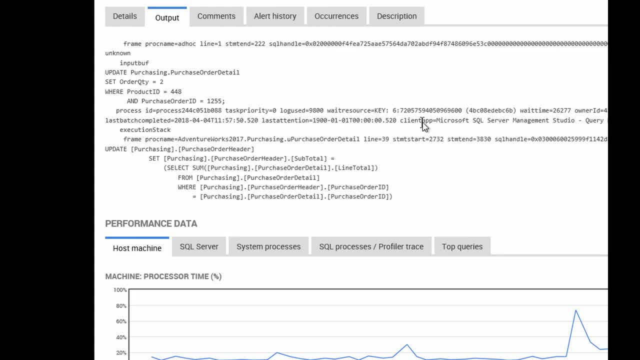 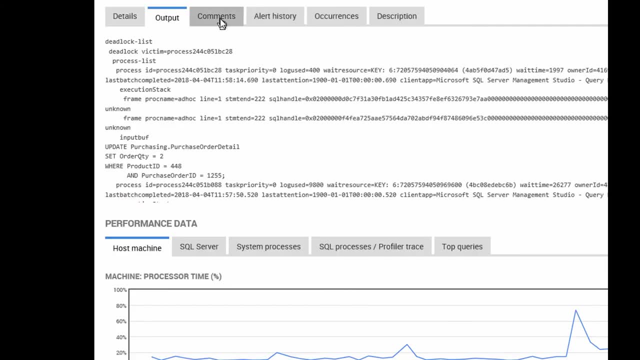 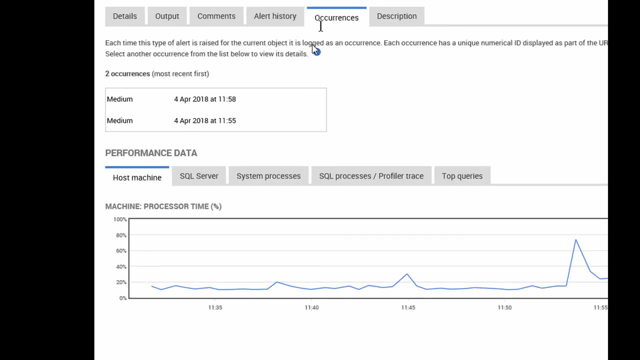 so you can have the full deadlock graph if it's needed. so you've got all of the information available to the deadlock itself. comments: if we've added comments, alert history. so the number of times this was, you know, occurred. we've had two occurrences today and the full. 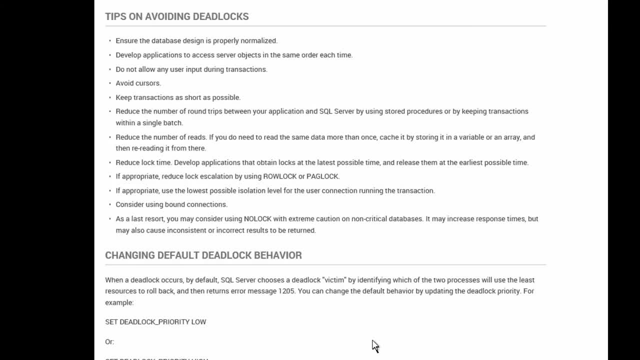 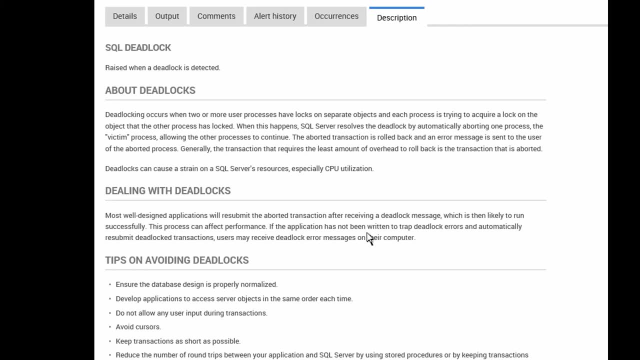 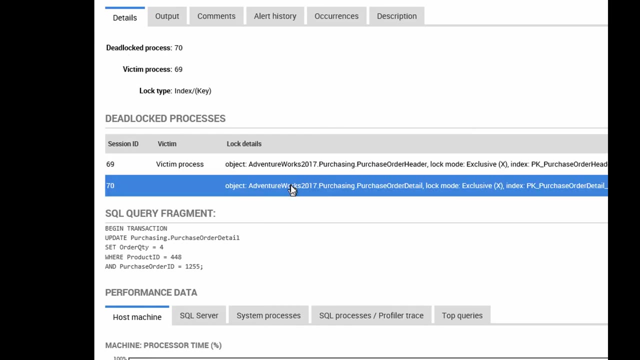 description of what deadlocks are, how to avoid them and how to how to deal with them. so everything you need to know to track down and fix this deadlock is immediately available right in front of you here, with with the information that we know that this is coming from this query and the other is. 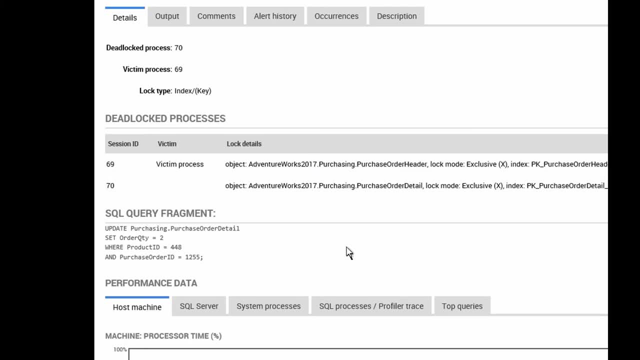 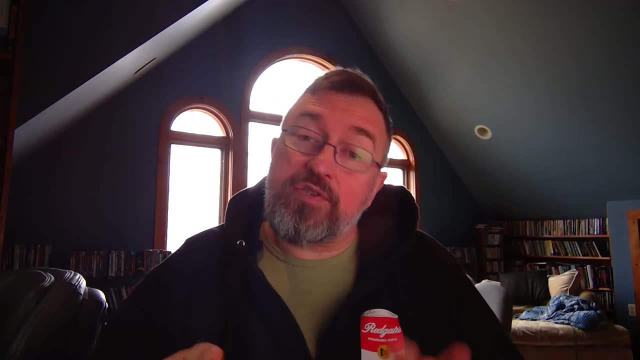 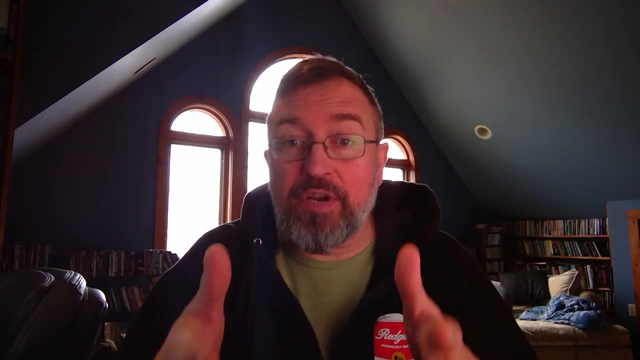 coming from this query and we know how to track down these deadlocks now because we've got the stuff to deal with it. alright, so now you see how to capture deadlock, see what they are, get alerts on them, drill down on the details of them and figure out what do we do to solve.